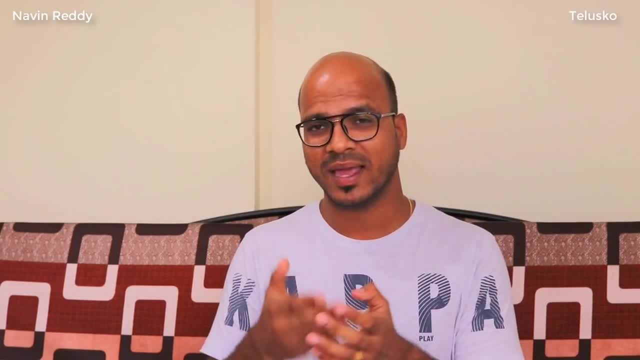 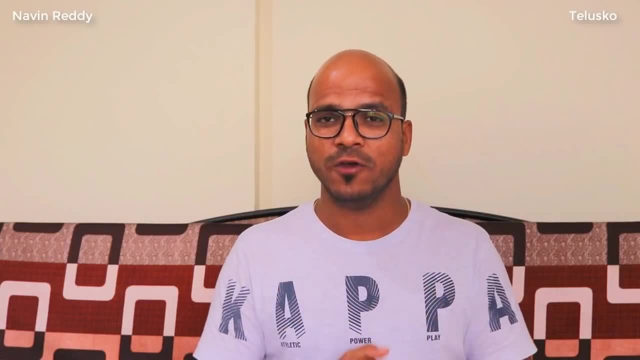 might change or maybe there is some miscommunication. So client is asking for something else and you are giving something else. So you need that continuous feedback right, and that's why we are using a different approach nowadays, which is agile. So, in agile, what you have, what you are. 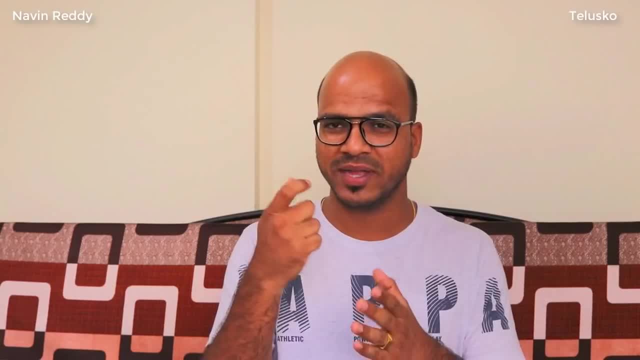 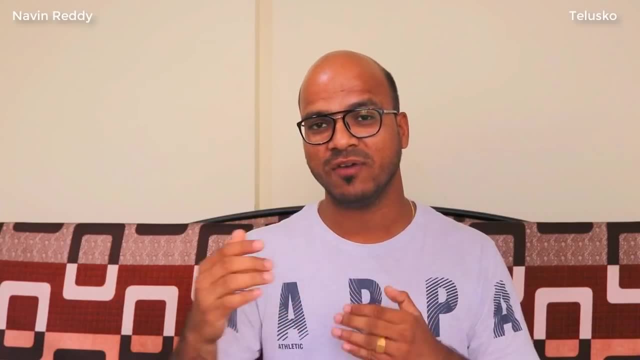 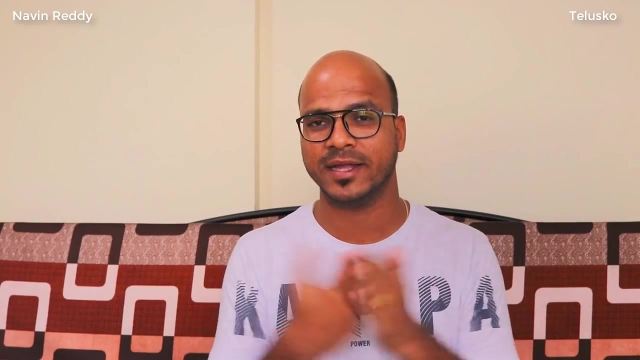 responsible is to give your client a ready product in every two to three weeks. Okay, not the entire product, but then the parts of it. So let's say, if you have 10 features, you can give one feature in two weeks or three weeks. Now, that will be amazing from a client side because you will get a 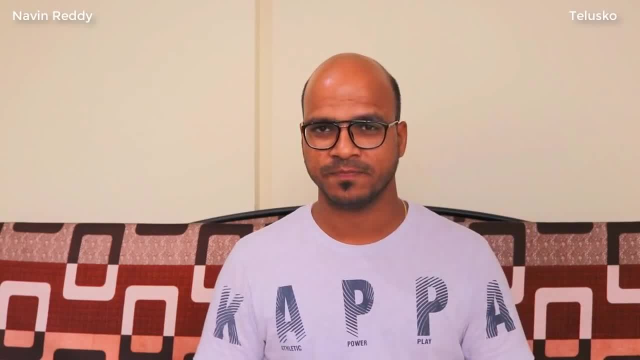 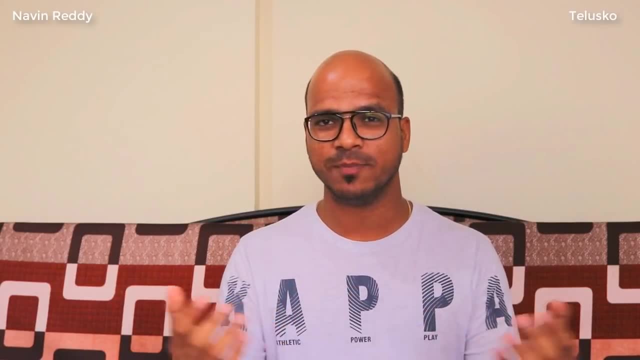 lot of feedback. Okay, that's one thing. So we have one thing which is agile. The second thing here is now. let's imagine you're working on a project and in that project you have certain modules and you have multiple developers to work on it. So what you have done is you have given one module to each. 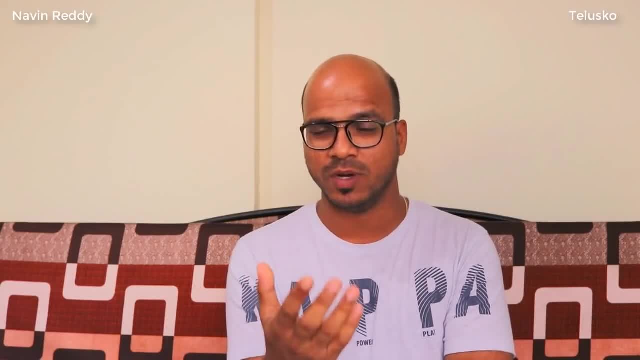 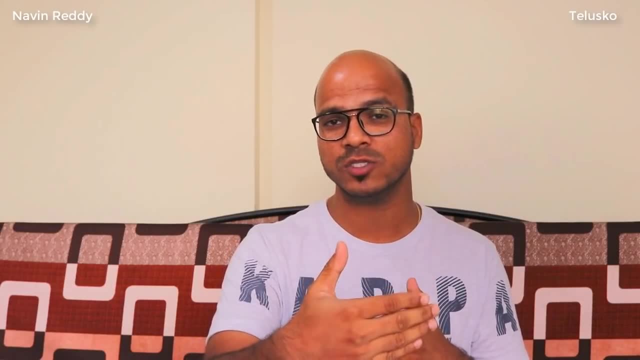 developer. Now the thing is, when you, as a software developer, work on a project, let's say you are using java here, so you will write a java code and you are also responsible to test it, and for testing you will be using junit, right? So you will be using junit and you will be using junit and you will be. 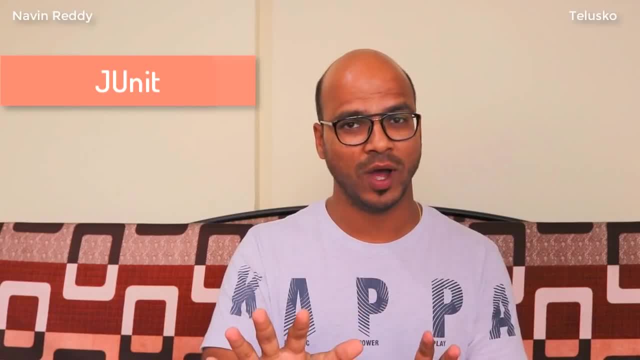 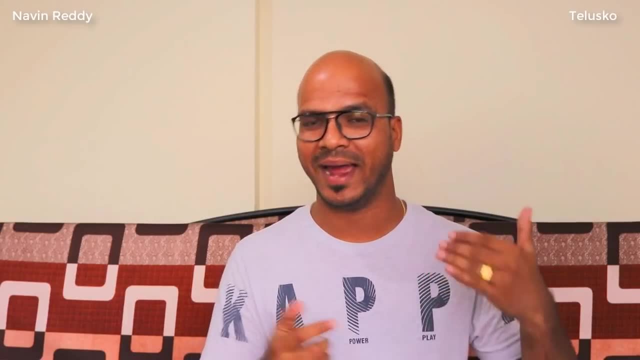 using java code right Now, when you test your class, it is perfectly working. so your unit testing is working perfectly. But then we miss one thing In testing. we have one more thing which is called as integration testing, because all these developers, they will work together right and when they work. 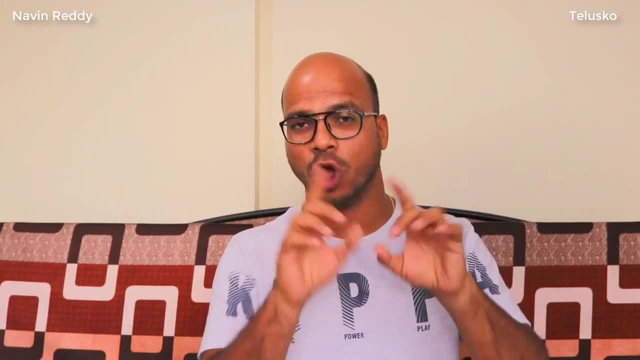 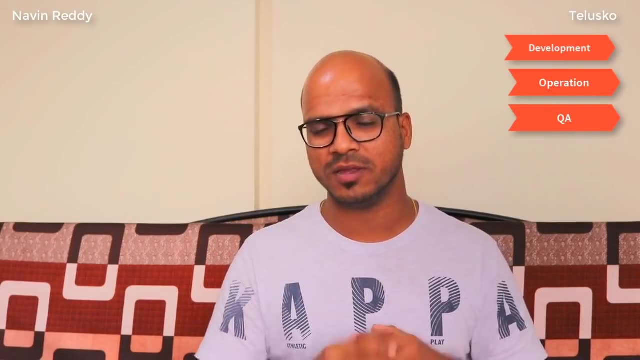 together. they have to integrate it somewhere so that your operation teams- because we have development teams, we have operation teams and we have a qa team, Now your operation teams are responsible to you know- take that project and deploy it on site. So you have to integrate it. 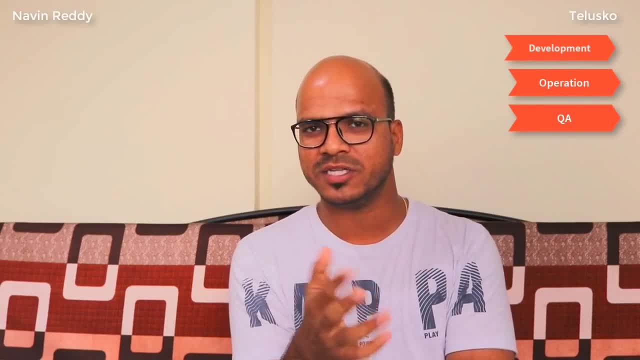 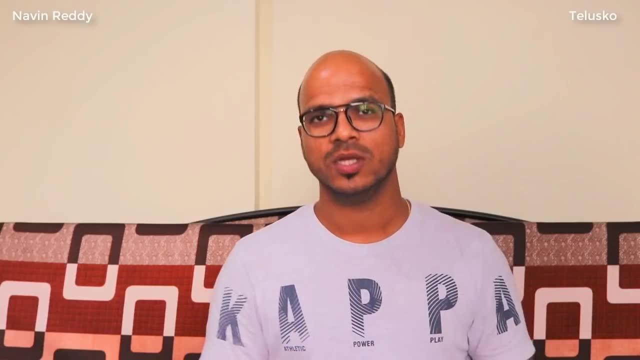 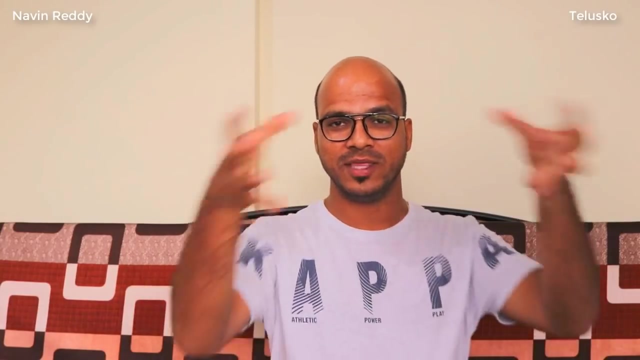 on the server, But then you have missed that integration testing, right? Who is responsible to do that? So what we have is: we have this automation test things. So let's say, this is Friday evening and you have decided: okay, so we'll work for one week and every Friday we will deploy the project, we will integrate. 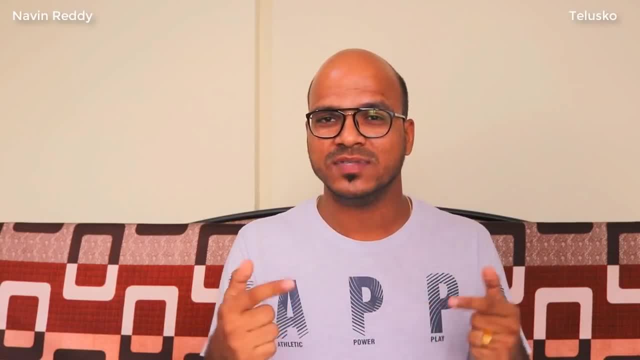 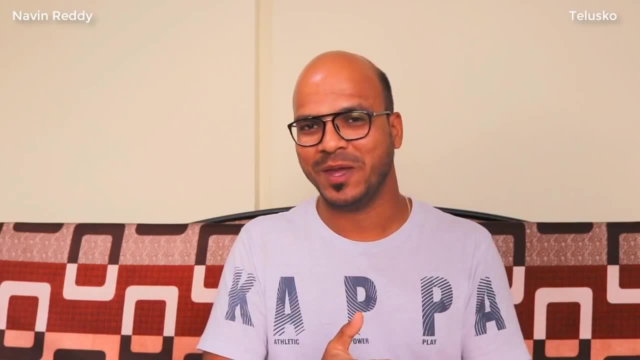 the project, and then there will be an automation test. What if something goes wrong in the automation test? What if there are bugs? Now the problem is: this is Friday evening. you don't want to spend your weekends in the office, So what? what you will do is you will solve that problem. So that's one. 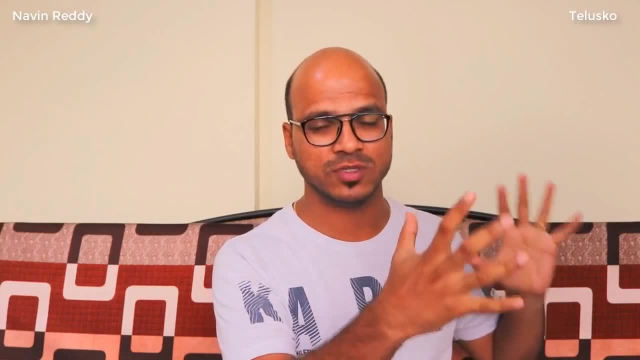 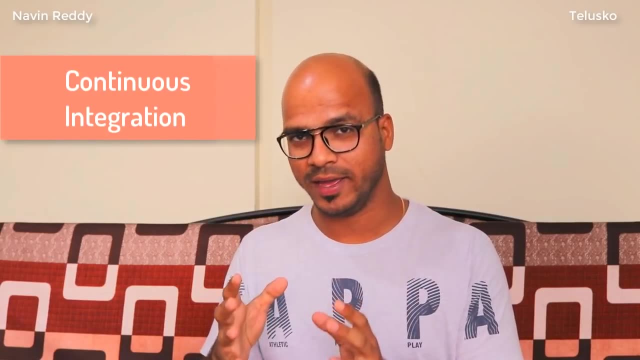 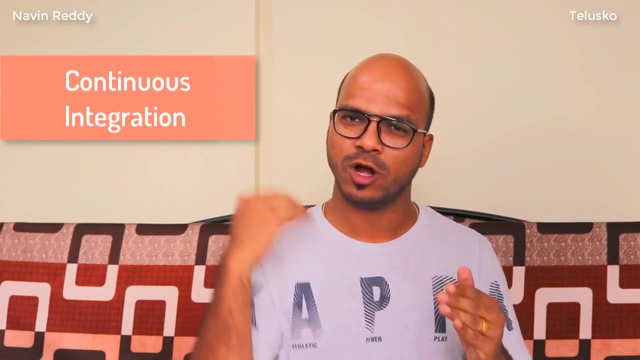 problem right? You cannot. you, you don't have to wait for an entire week to submit your project, because that happens in the industry. To solve that problem, we have a concept of CI. Now, what CI stands for is continuous integration, As name suggests. what if you integrate your modules? it's. 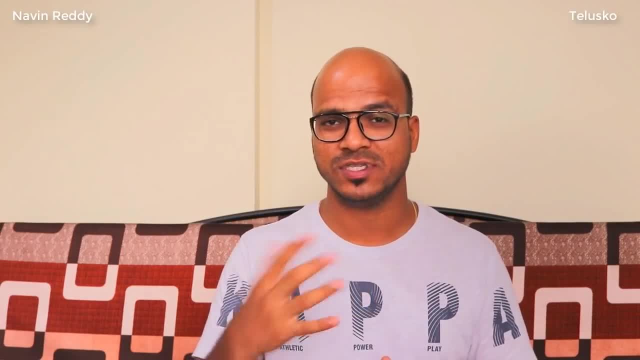 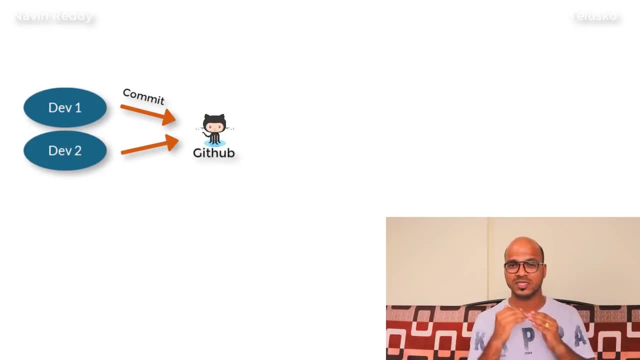 very often. let's say, in a day you will be doing maybe five to six commits, right? So every time you make a change, every time you think it's going to be a problem, you're going to have to do a test. So let's say it's working for you in your unit test, just submit it, or just commit it on the. 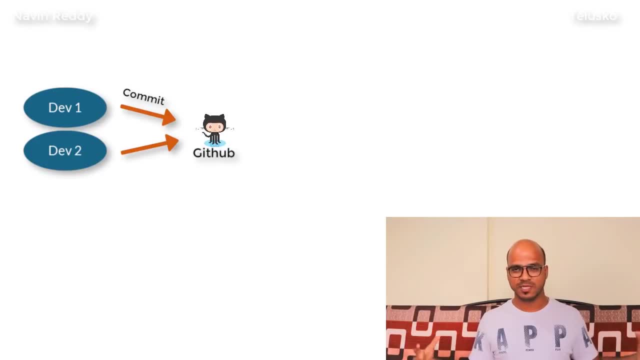 share repository. The advantage would be, let's say, if you have five developers, all these people will be committing to server and every time you commit there will be an automation test. That means write, commit and test right. So at the end or after every commit you will be having a ready project. 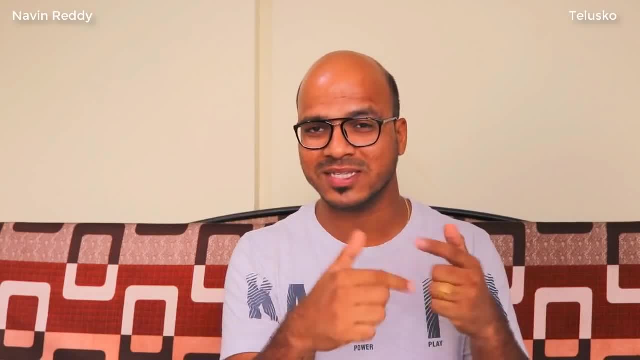 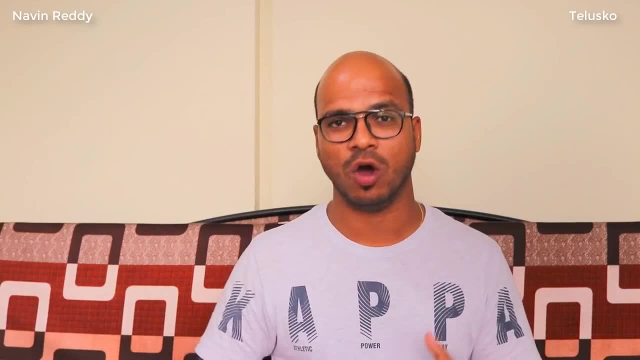 which is tested and you have the confidence that it is working because there's a test happening behind the scene, right? So that's the advantage of CI. CI simply means, instead of committing at the end of the day or maybe after a week, just the moment you have done the code, the moment you you think it's working for. 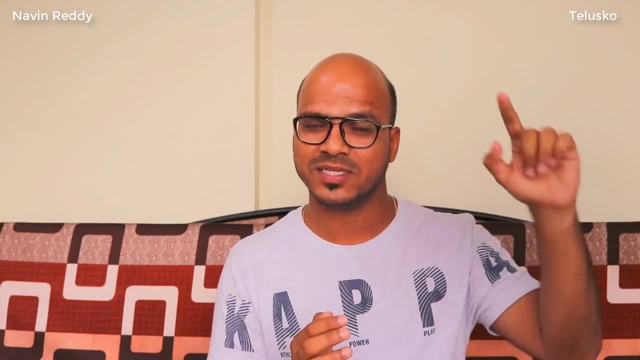 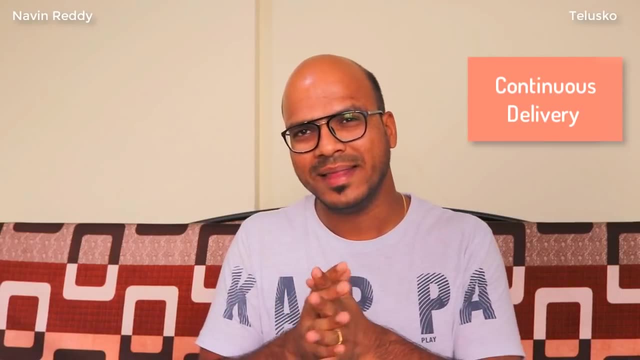 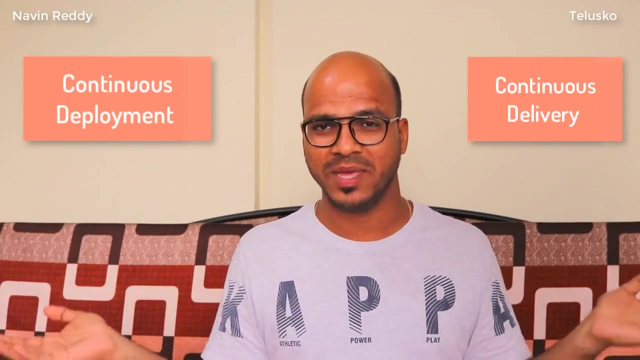 you in a unit test, commit it so that it will be test. it will be. there will be automation test done on the server. After this we also have a concept of continuous delivery. Now, in fact, we have CD. we have two parts in CD. We have continuous delivery and continuous deployment. Now, people often mix. 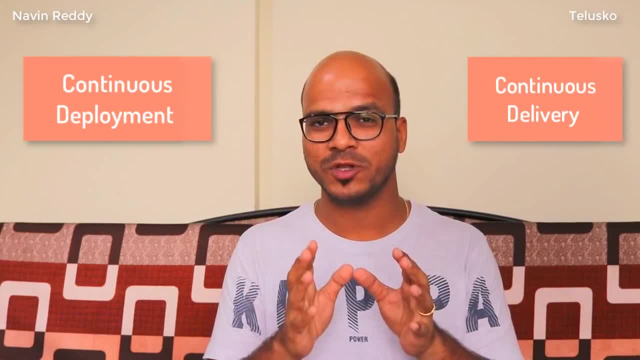 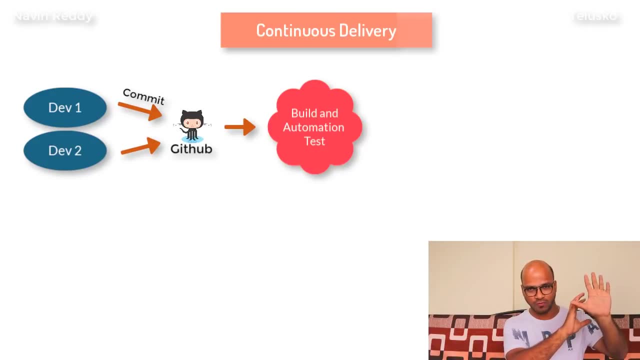 those two terms, but they are not same, They are different. They are different, They are different. Okay, so it's important to understand the difference between delivery and deployment. When you say continuous integration, you have the project you have you are committing. very often, right Now, it is possible that your commit your the entire repository after the. 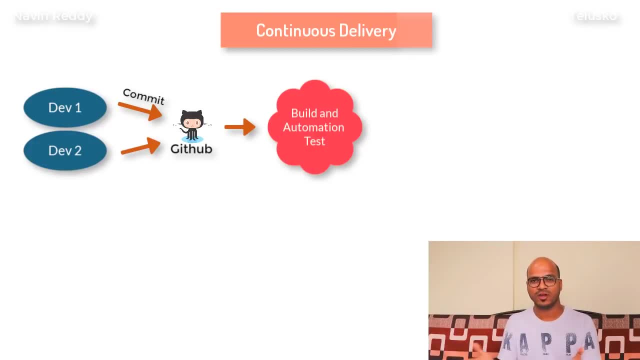 committing is ready for delivery, Maybe after. if your client says, hey, we want to see what's our progress, You can simply show them the working model, not on the production server, of course. You will be showing that on a mock server, So you will be getting a production like server. 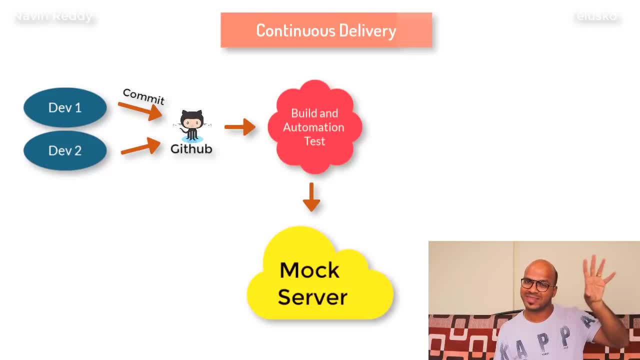 a fake server and you will run the current project on that server right. So it will give you the confidence that things are working and it will also make your client happy. Plus, you can also check for the performance of the system. So when you shift your project from this thing to 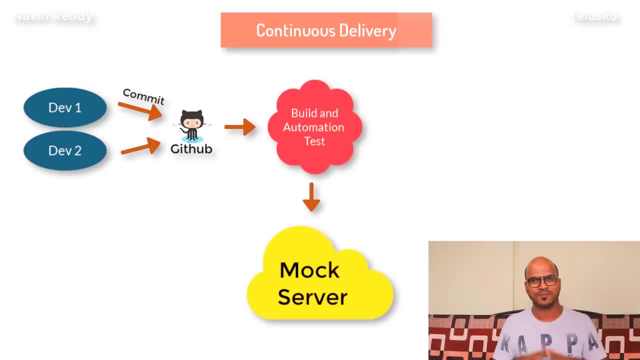 your production environment, how it will, so you can mimic those things right. So that's a delivery. okay, continuous delivery. So of course you will not be deploying it on the production server, but you are keeping it ready for the deployment. So at any point you can, you can think. 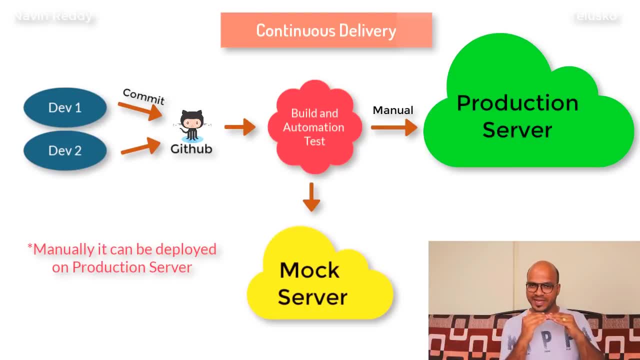 okay, let's deploy it, and it should be available for that. So integration is: you are pushing the code, delivery is making it available for deployment. Now, what about continuous deployment? Now, continuous deployment is a bit scary because when you, the moment you commit your code after the 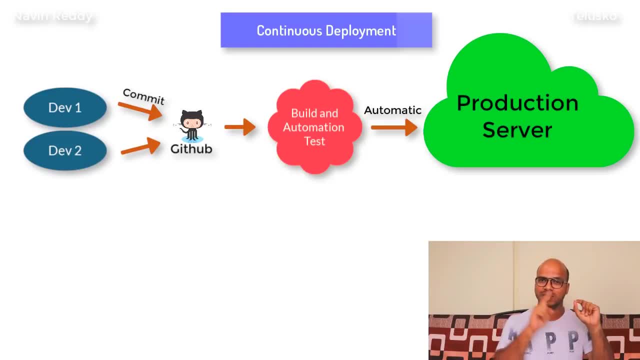 automation test, your code will be directly deployed on the production server. okay, If there's something wrong you're gone, but then it doesn't happen very often, right? So you write a code, you commit it and be first you test it, Then there's automation test and then it goes to the production server. That is continuous. 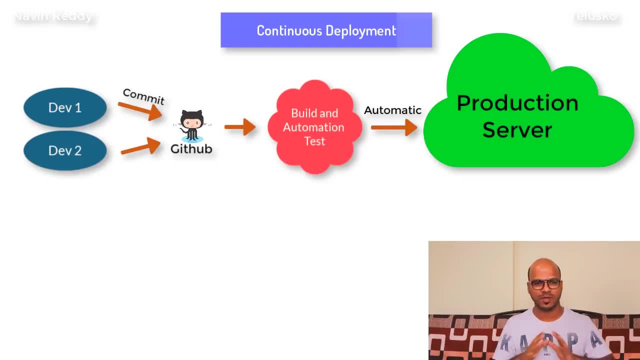 deployment. Now, not every company do this. okay, because every company they have different requirement, they have different approach. Some companies only go for CI. they don't go, they don't even go for CD, because some company go for delivery and some company go for continuous deployment. The moment you commit, it will keep getting deployed and I mean it will be. 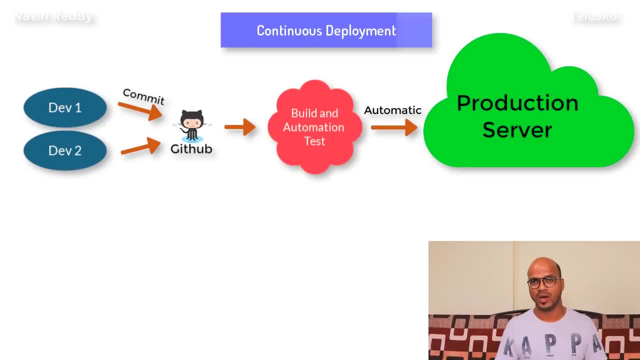 tested and then it will be deployed. Example: people who are working with microservices. they believe in continuous deployment. and there are some big companies like Facebook. they are doing this: Write the code, commit and it will be deployed on the on the server. So that's CI CD. 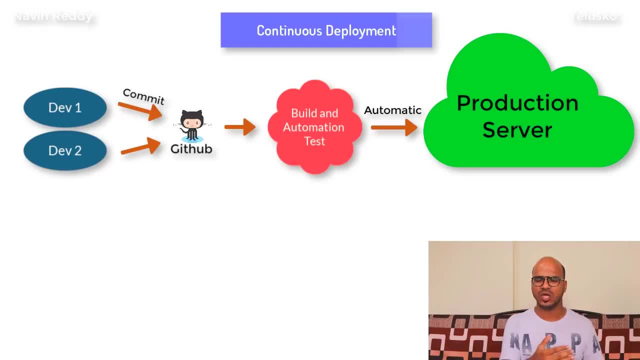 Now, is it that easy to implement? the answer is no, because initially, you have to, you know, you have to make your team ready for this. Second, you have to get a pipeline so that it will, everything will happen in the in the sequence. So, because you will be committing it, you will be testing. 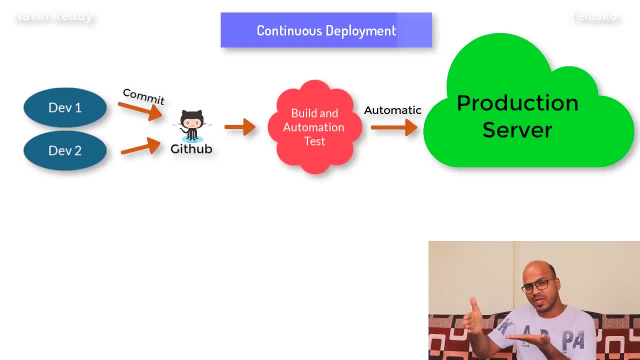 it and then it will be going for deployment. So that's a code pipeline which you build. Now there are different tools available for this. We can use Jenkins, which is one of the best tool available, or if you're using AWS. in fact, in the description area, you will find a video of mine. 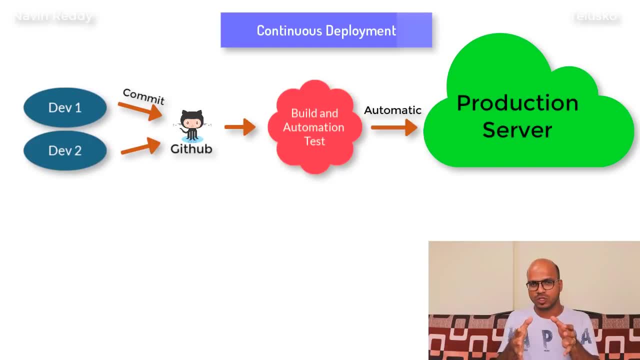 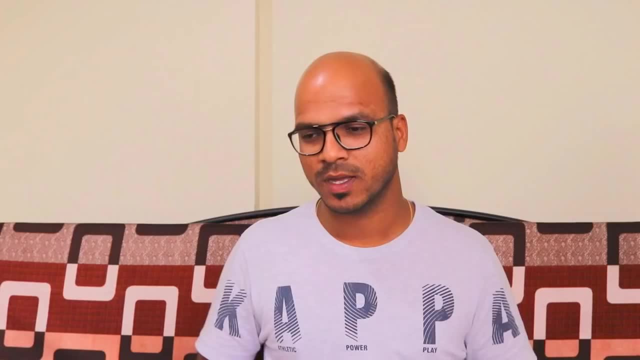 which explains all this concept. okay, Now, the main focus was not to explain CI CD, but I was trying to explain AWS. but you can match it up right how exactly things happens in the real world. So that's what is CI CD is. So in case, if you are going for a DevOps job, this is very important.